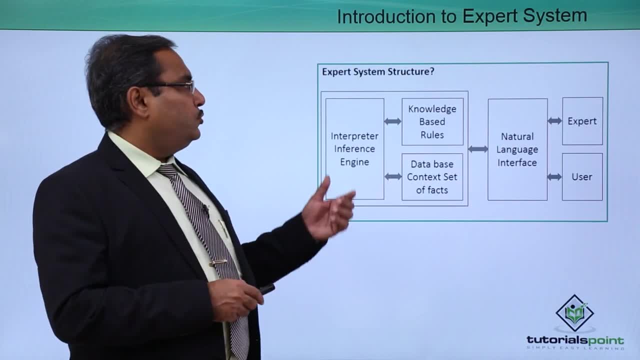 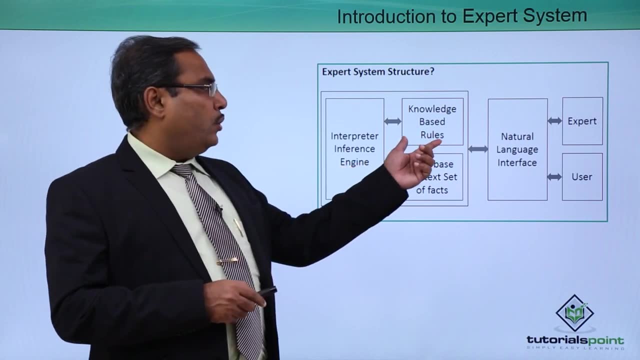 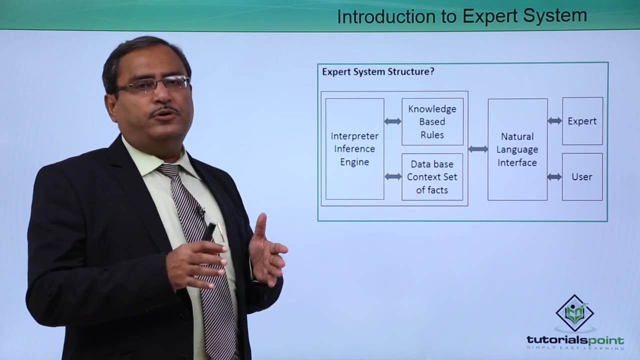 each and every component separately now. so at first we are going for this diagram. so this is our interpreted inference engine: knowledge base, rules, database, context, set of facts. so whenever we are having some facts which will be denoting data, we usually call it as a database. and whenever we are having 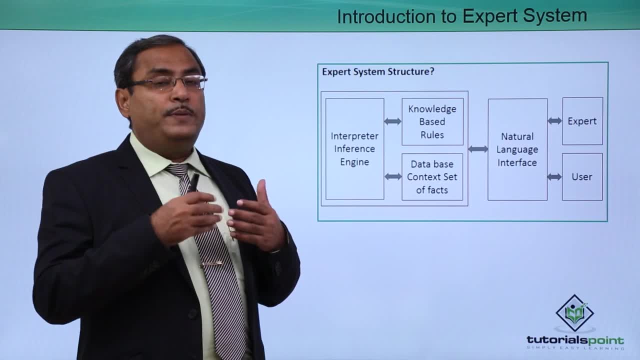 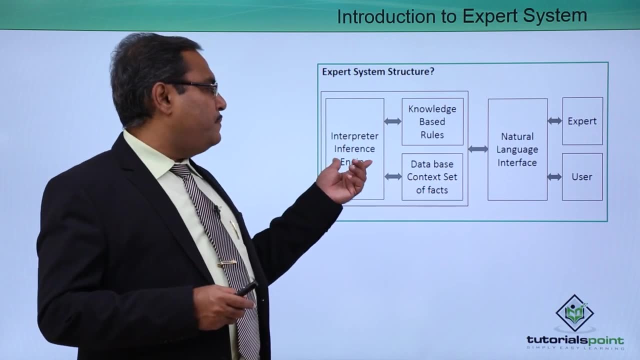 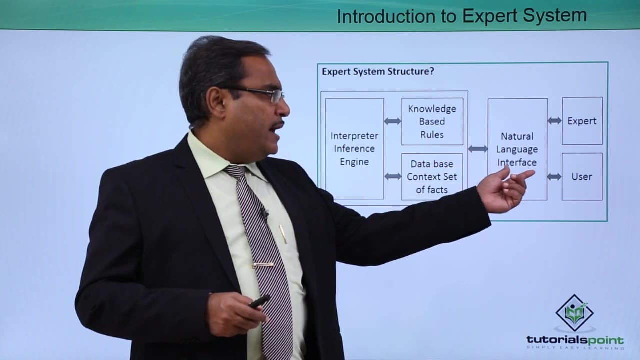 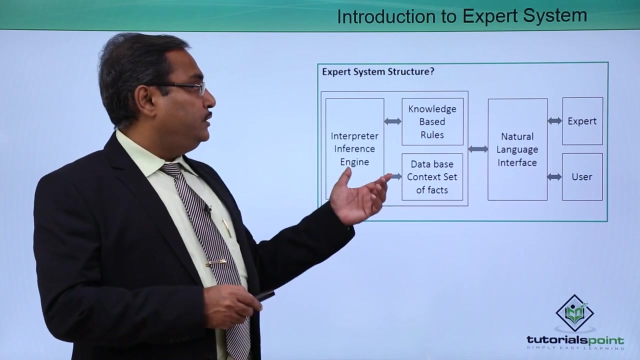 some rules containing if and then part, then we will be considering them as a knowledge base. with this knowledge base- rules and database, context set and interpreted inference engine, with this whole, this natural language interface will be interacting and with this the user will have its interface and also experts can interact with this expert system. so this 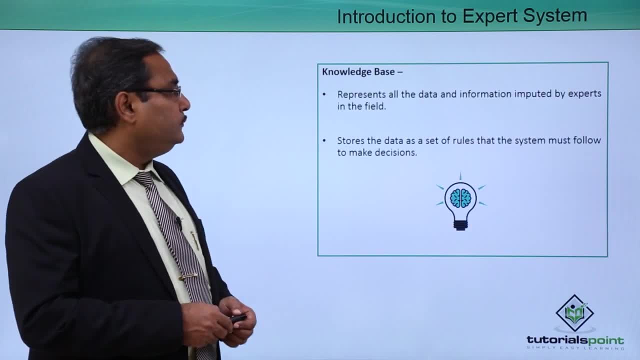 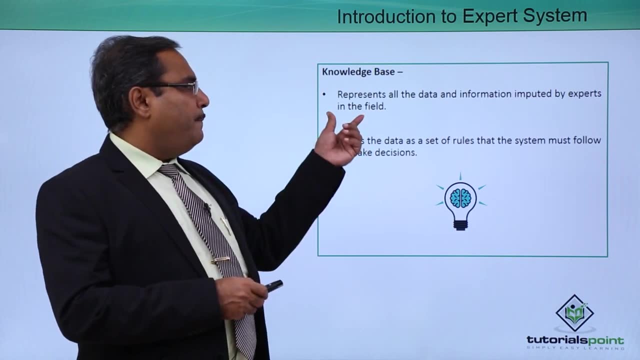 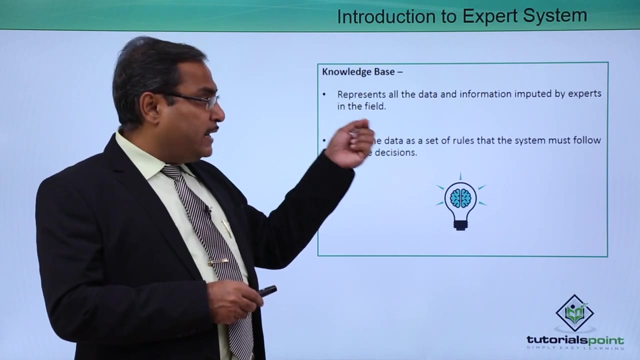 is the expert system structure. so at first we are going to discuss the knowledge base. represents all the data and information imputed by the experts in the field. so this knowledge base will be actually representing the data and information which will be provided by the experts. stores the data as a set of. 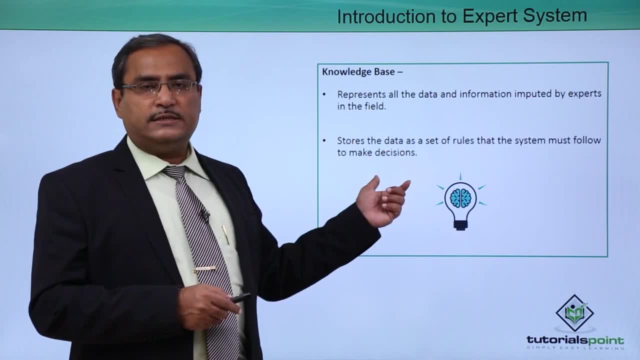 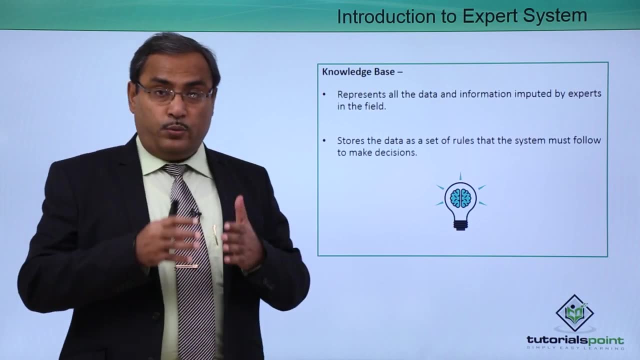 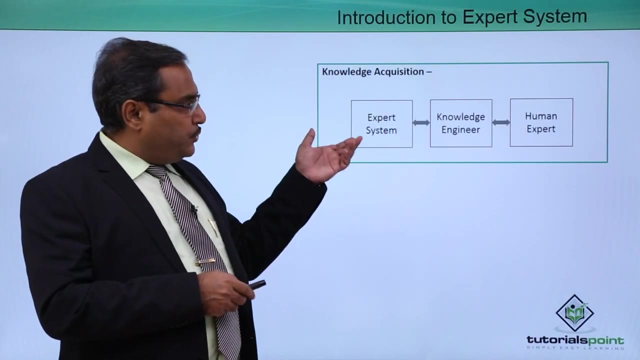 rules that the system must follow to make decisions. so that means it will store the data in the form of rules that the system must follow where we are supposed to take some decisions there. so next part is our knowledge acquisition. so here we have given this diagram to 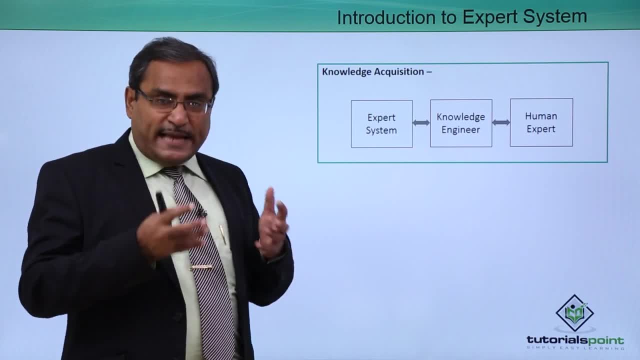 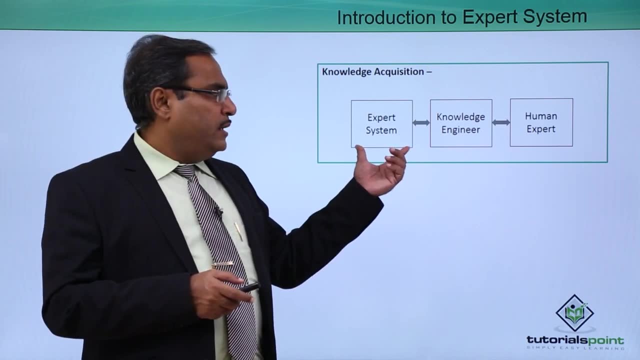 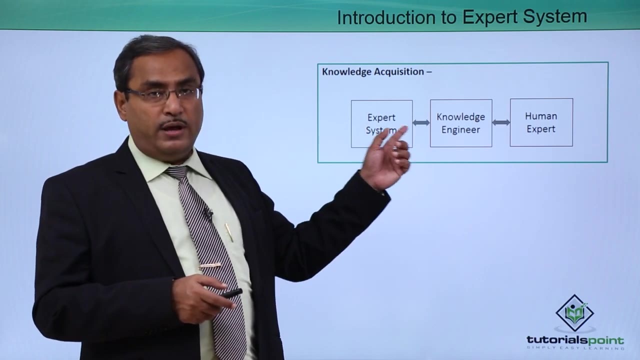 depict what is a knowledge acquisition and how this acquisition- that is, accumulation of knowledge- will take place. so here we are having component like expert system and here knowledge engineer and human expertise. here this knowledge is having a bi-directional flow in between. so this expert system will get the knowledge from knowledge engineer. 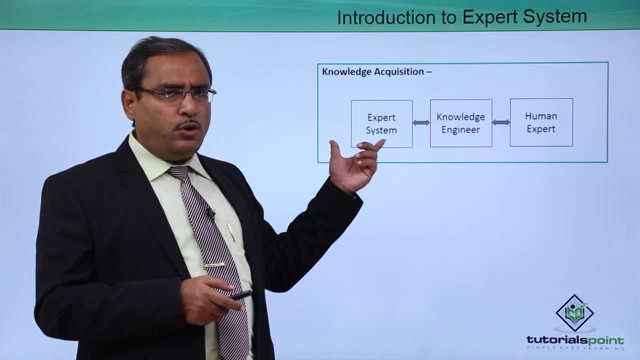 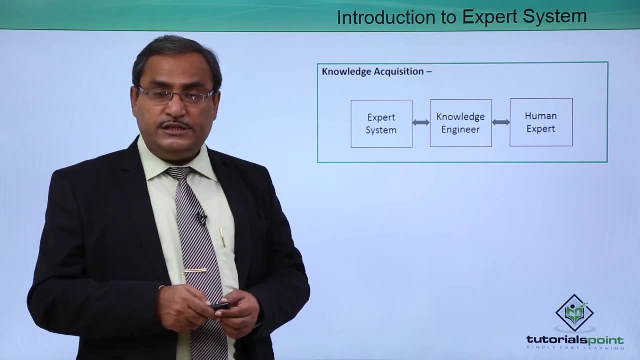 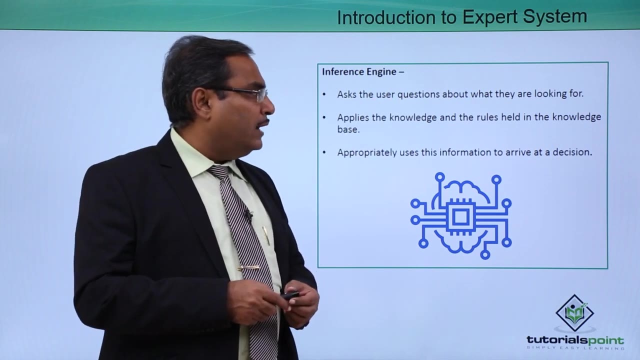 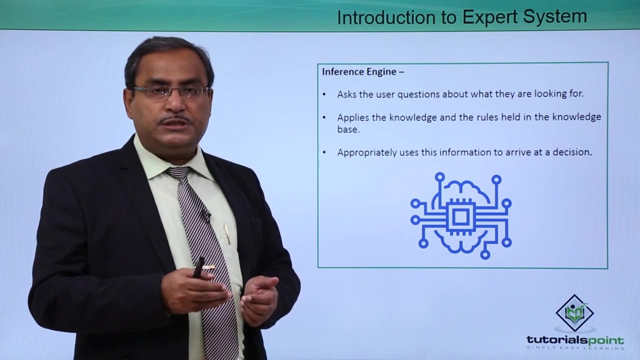 knowledge engineer can also access the information and knowledge from the expert system, and there are. the human expertise are there, so they'll be also interacting with this knowledge engineer module inference engine. ask the user questions about what they are looking for. thank you, so the process of quad should be taking. the queries will be taken. the